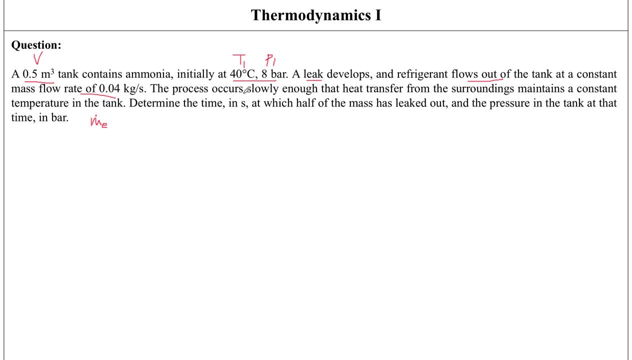 And what? what's it telling you is that the process is going on slowly enough that you've got a constant temperature in the tank. okay, so it's a constant temperature process. So, basically, T1 is going to be equal to T2, and what you need to find out is: you need to find out the time in which half 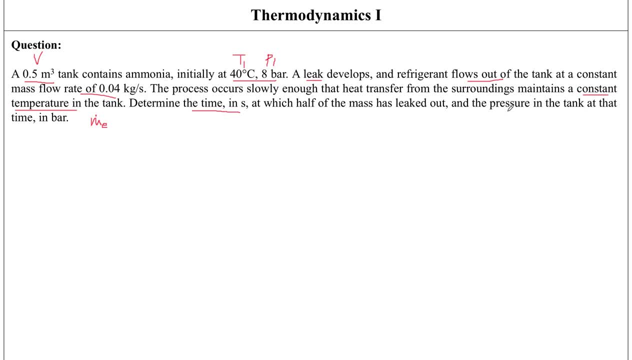 of the mass. so half of ammonia has leaked out, and the pressure in the tank at that time okay. So you've got a tank and this tank has got ammonia in it, you've got volume given to you and then some kind of leak is developed. so you've got mass flowing out of the tank and you've 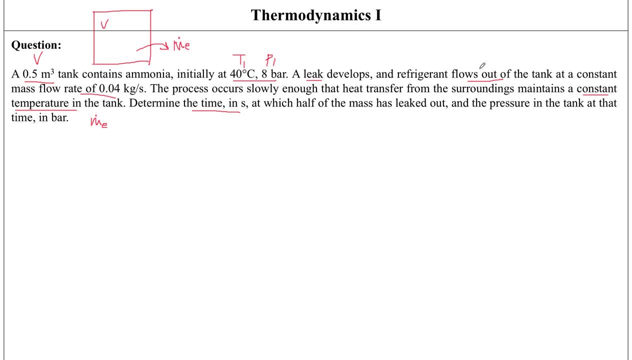 got the mass flow rate given to you as well. Okay, so if I was to try and make the PV diagram of it, I wouldn't be able to do that right now because I don't know where exactly. does it live within the dome? Does it lie outside? 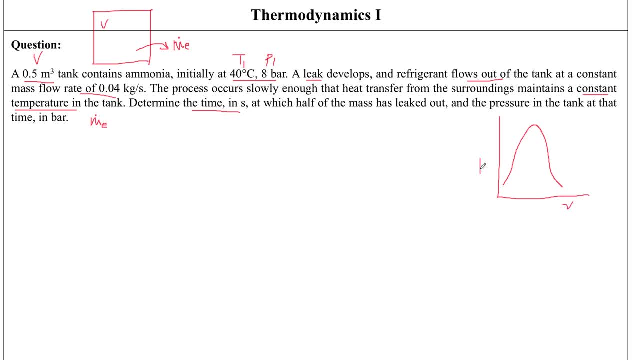 of the dome. So if I was looking at, let's say, the PV diagram, it, and then I would have constant temperature lines over here. okay, so I don't know if I can spot where the first state is, because I've got pressure and temperature given to me, but I need to find out whether it's a mixture, a liquid. 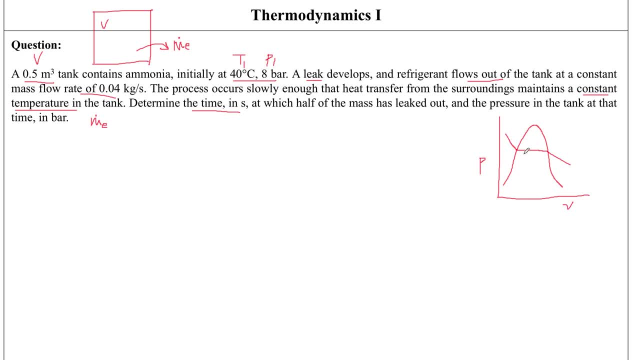 vapor mixture, whether it's a superheated vapor, whether it's a compressed liquid. so that is something that I need to do from the tables. before I do that, I can go ahead, because we're analyzing a control volume right now. and why is it a control volume? because mass can flow into and out of the system. mass is 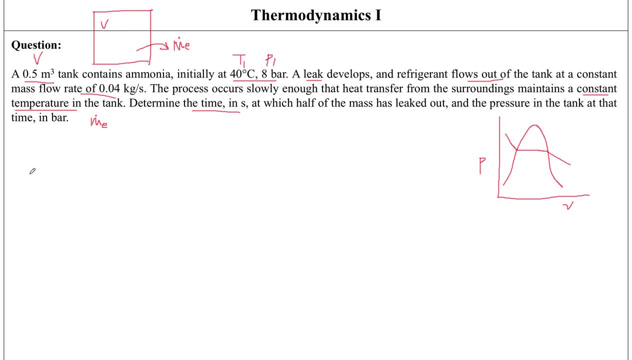 flowing out of the system right now. so that's why it's a control volume. so if I apply the mass balance equation on it, which is gonna be this one- basically change of mass according to time- it's gonna be equal to mass flow into the system: m dot I minus mass flow flowing out of the system, because we've got no mass. 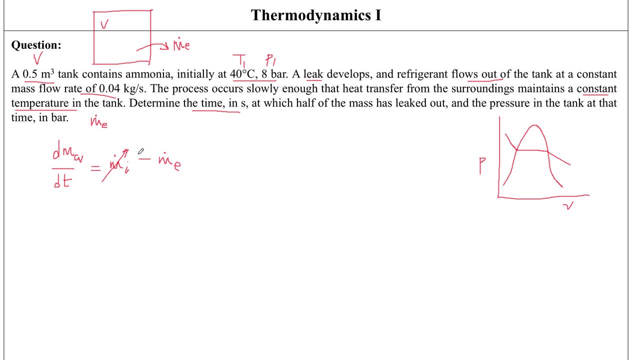 flowing into the system, so this is gonna be zero, but obviously we've got this happening. mass is changing within our system with respect to time, so this is gonna stay. this is gonna stay as well, and this can basically- I can write this as if I move DT on to the other side- it's gonna be equal to. 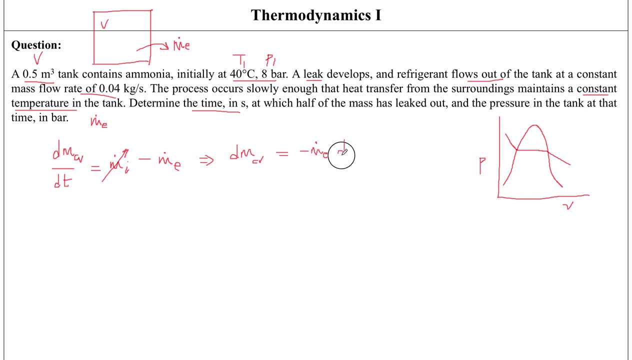 minus m dot into DT, and now I can apply an integral on both sides. right, so I can apply an integral on both sides. it's gonna be from mass of the control volume at time zero to mass of the control volume at some time T, and we need. 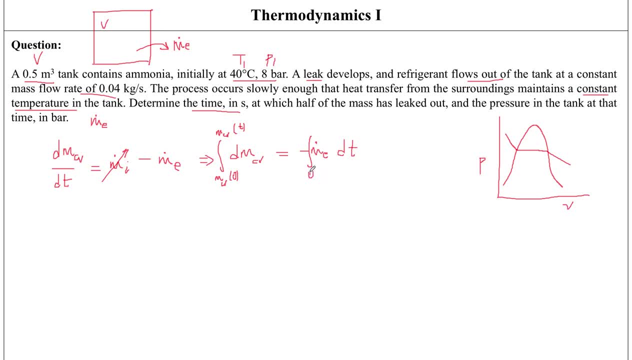 to determine that, and over here it's gonna be again from time zero until T, and now we can just apply this integral on both sides, and if I apply it on this side, I simplify this integral. it's gonna. I just have to put these limits in and 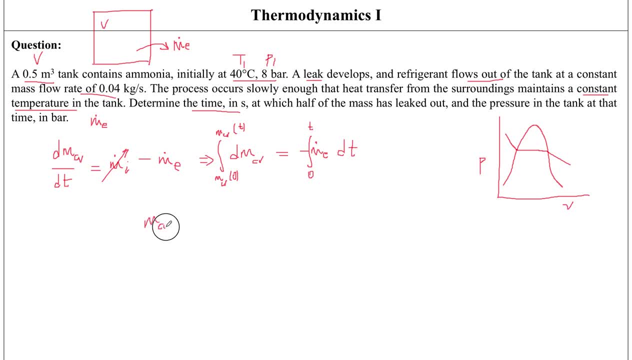 it's gonna be mass of the control volume at time T minus mass off the control volume at time zero and that is gonna be equal to minus, because me is constant. okay, it's a constant mass flow rate. so I can just move this out. and what's DT gonna be when I simplify this integral. 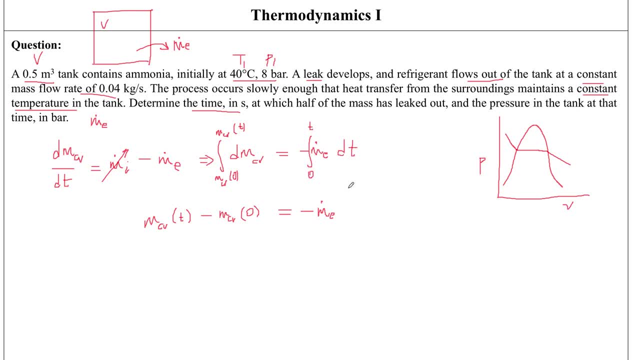 DT over time: zero to zero to T. I simplify this. it's just gonna become T and then I can plug these in and it's gonna stay as T, because this is gonna go out so M dot and two t. or if I substitute m dot e exit mass flow rate, here it's gonna be minus 0.04. 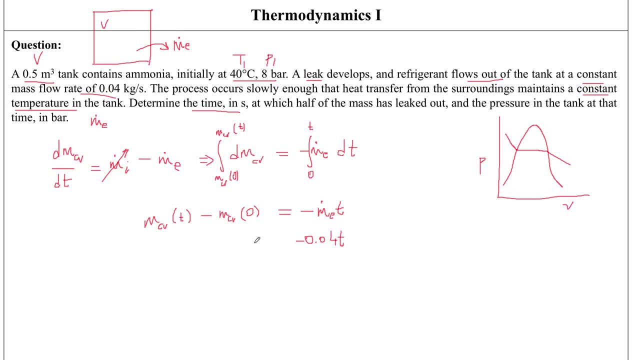 into t, okay, and now I can basically write this entire thing in terms of t, because that is the unknown, okay, and that's gonna be mass of the control volume at time t minus mass of the control volume at time 0, divided by 0.04. 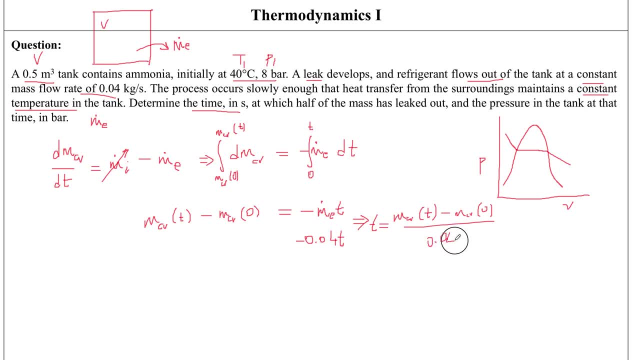 okay, I've just simplified this entire thing. you can try doing it yourself as well. and now I can work out the mass flow rates at time 0 and t, so the mass flow rate. I'm sorry, I can work out the mass at time 0 and t, so the mass at time 0. 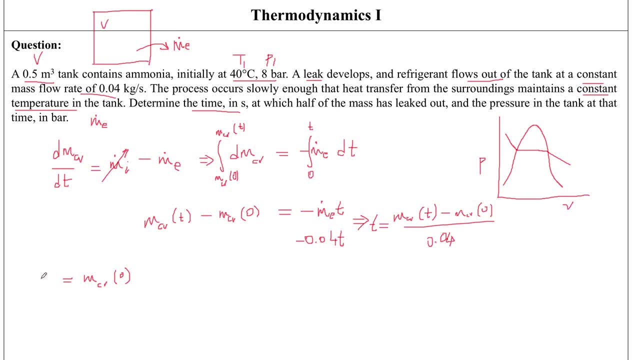 is gonna be. basically it's our initial mass. so mass at 1- and I can find this out because I've got volume given to me, I've got initial conditions given to me at state 1, so from the relationship of specific volume and volume, mass is equal. 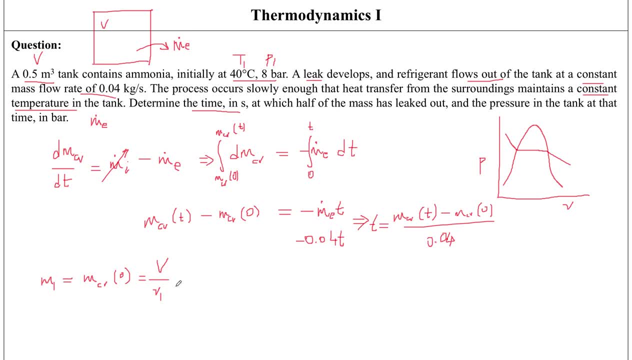 to volume by specific volume at that state. so, using these two, I can go to a tables for ammonia and I can find out the value for specific volume. okay, so I'm gonna leave that as an exercise for you. how are you gonna do that? I'm just 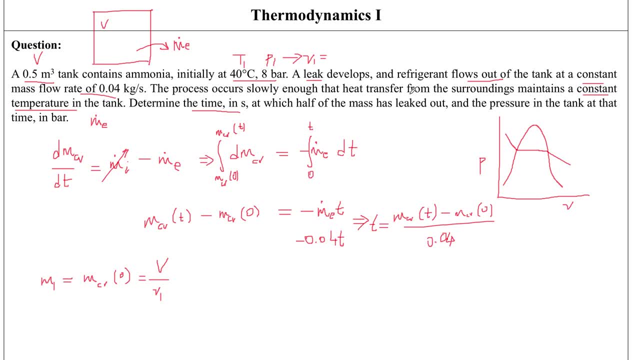 gonna give you a hint: it's a superheated, it's in, it's gonna be in the superheated region, but you're gonna have to figure out why it's in the superheated region based on the pressure and temperature information given to you. so this is: 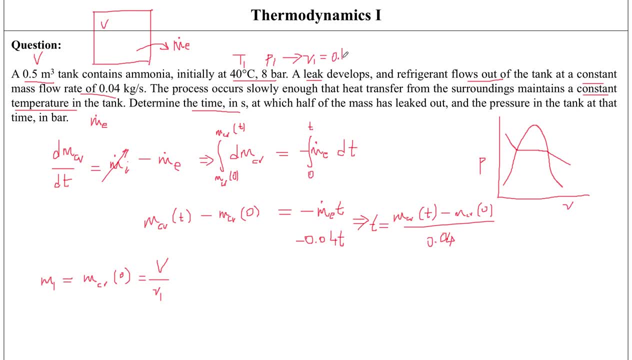 gonna be point one, seven, seven, two meter cube per kilogram. okay, so now you got volume and you got to this specific volume as well. just plug that in and you're gonna have your mass off the control volume at time zero. and it's gonna be two point eight. 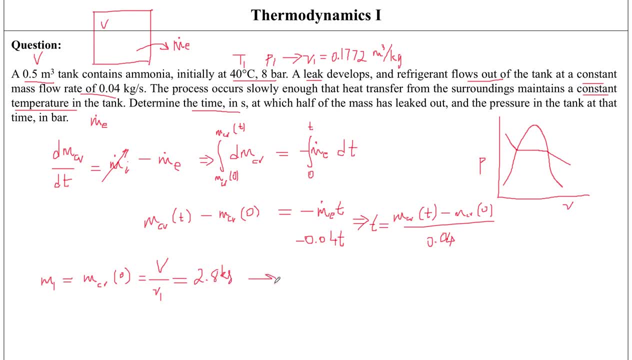 kilogram round about that and from here you can also now find out- sorry this is, you can find out the mass at the second state. and how can you do that? because it's telling you that you need to determine the time in which half of the mass has leaked out. so that means m2 is going to be half off m1 and one by. 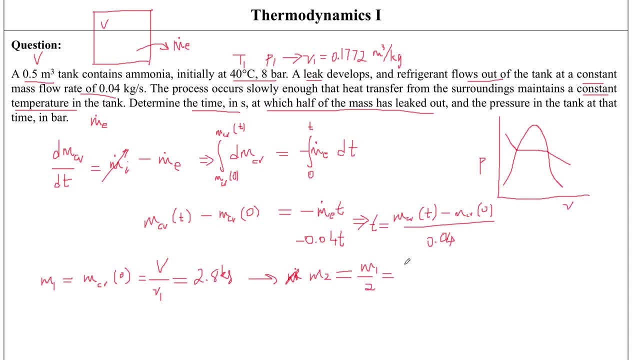 two, that's just gonna simply be two. point in eight by two, I'm gonna get 1.4 kilograms. okay, so now that you've determined these two, you can plug them in into this equation over here and you'll be able to find out the time that it takes for the. 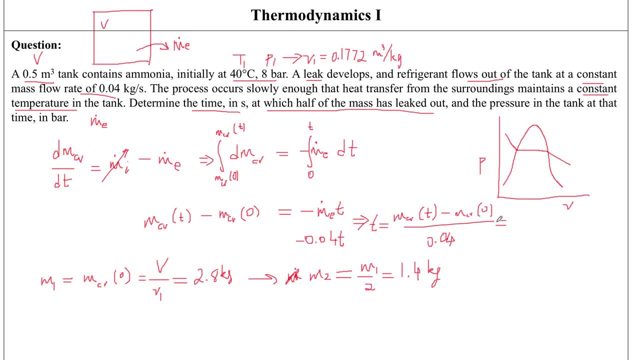 mass to leak out, and that's gonna be around about 35 seconds. now that you've found out the time as well, you can go ahead and now find out the temp, the pressure in the tank at state two. and how are you gonna do that? again, you're gonna use this same concept. 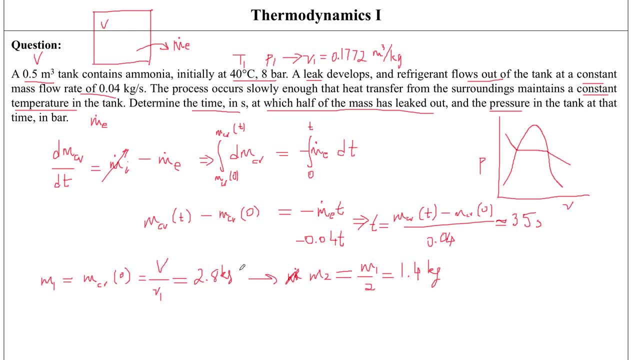 because you know the volume and the mass at two. so from there, what you can do is you can work out the specific volume at two. right, it's gonna be volume divided by mass at two, and you're gonna get some value from here. let me write that down. 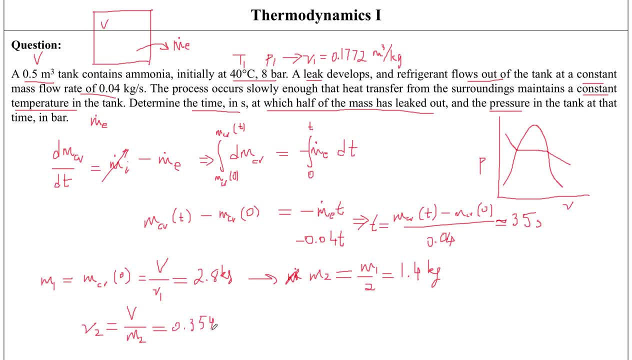 for you point three, five, four meter cube per kilogram. and now you can go ahead and look for this value in the table, in the thermodynamic tables and the table for ammonia. and I'm just gonna give you a hint again: you're gonna have to go to table a one, five in Shapiro's. 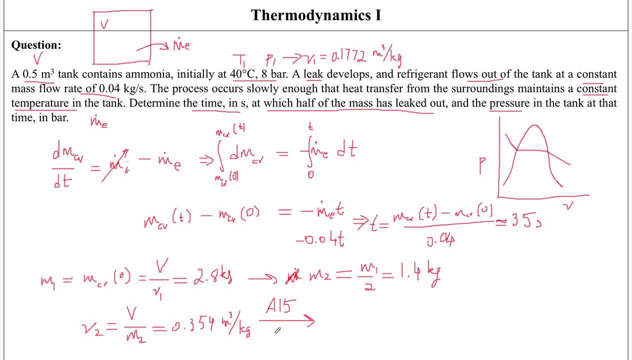 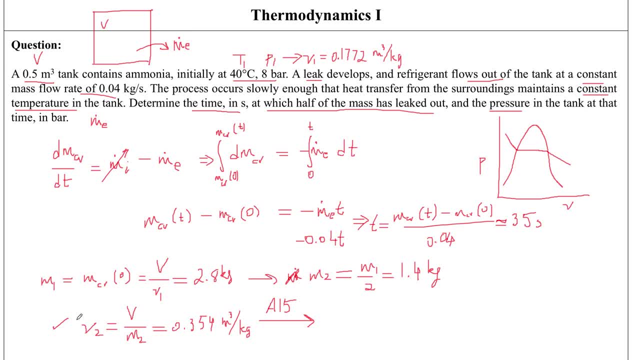 information that I mean information that you can use with the tables. you've got specific volume and two and you've got the temperature at two. okay, so using those two, you're gonna go and interpolate in the table and find out the pressure at state two and that's gonna be somewhere around four. point one: 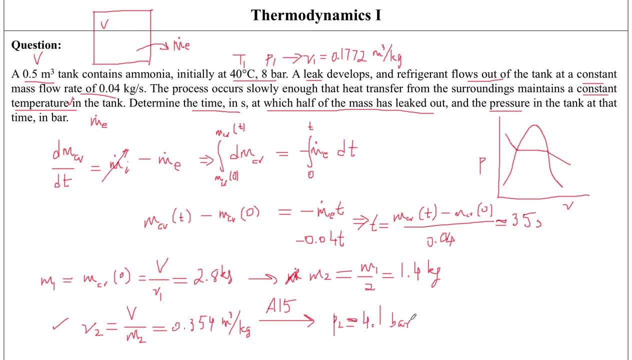 bar. so initially you couldn't make the PB diagram, you couldn't generate it for it. but now that you have all the information given to you, you're gonna be able to identify whether the pressure has increased, whether the pressure has decreased, whether the superheated ammonia has moved into the mixture region, whether it's still superheated. 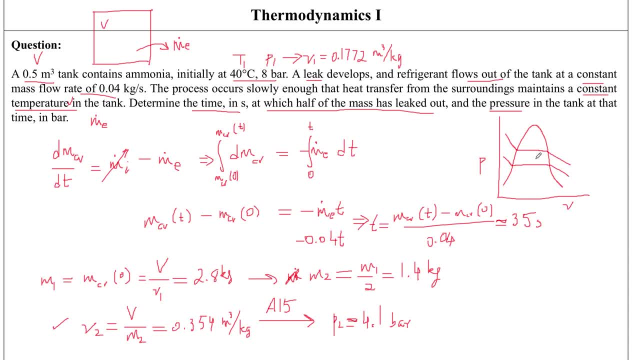 ammonia. so that is something that I'm gonna leave up to you. you can go ahead and play with that- this and find out and how it looks on the PV diagram, and also go ahead and try to make the TS diagram as well. Also, one more thing that you should do is use 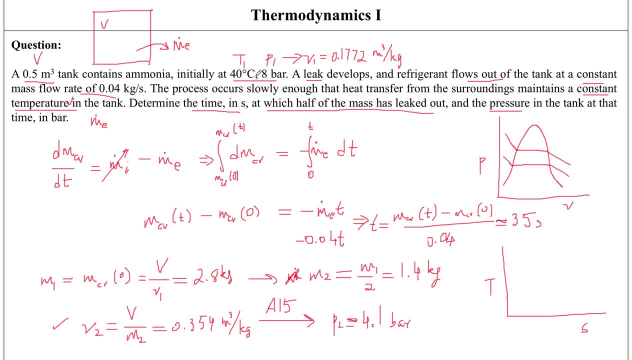 both tables because you've got pressure and temperature information given to you. so for ammonia, use the temperature table and the pressure table as well to find out the value for a specific volume at one. see how you're gonna be able to do that. that's gonna help you as well with reading the tables. 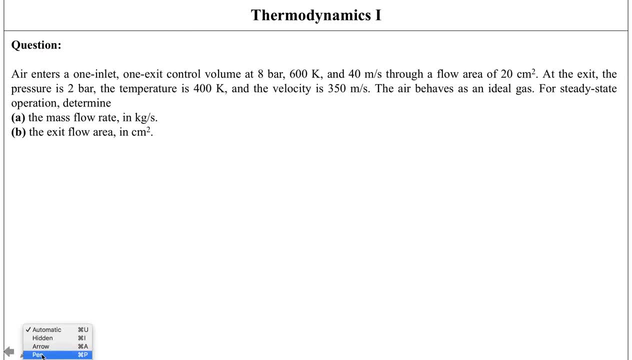 Moving on, though, I'm gonna go to the next question now and now you've got a case where you've got air that is entering into a one inlet, one exit control volume, and you've got information that is given to you at the inlet, at the exit control science which is going to give you some information, isn't it? 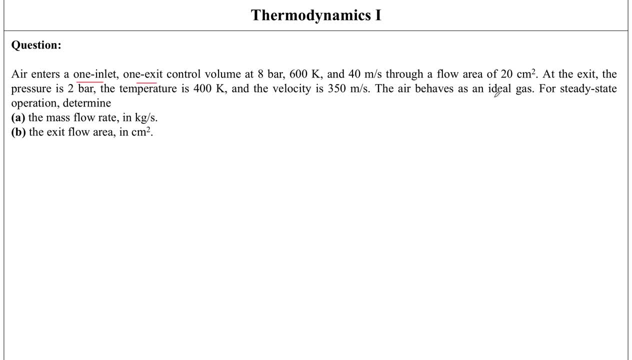 exit and you've been told that air is behaving as an ideal gas and, yeah, it's steady-state operation. So again, we're gonna start with applying the conservation of mass principle onto this control volume and that is going to be change of mass across the control volume according to time equal to incoming. so 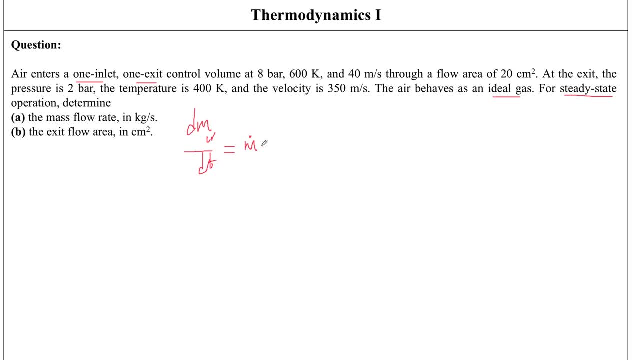 if there were multiple inlets, let's say there were two inlets, then it would have been m1 plus m2. but because we've only got one inlet, so we only got m dot 1 or m dot i you could say, and then you've only got one exit. so that is why you 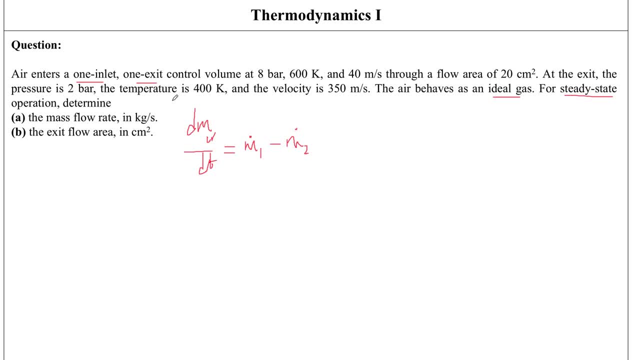 only write m dot 2, otherwise if there were two exits or outlets, it would have been minus m dot 2, minus m dot 3 or minus m dot e1 minus m dot e2. okay, so this is inlet minus outlet and because it's at steady-state, so this term goes out. because there's no changes. 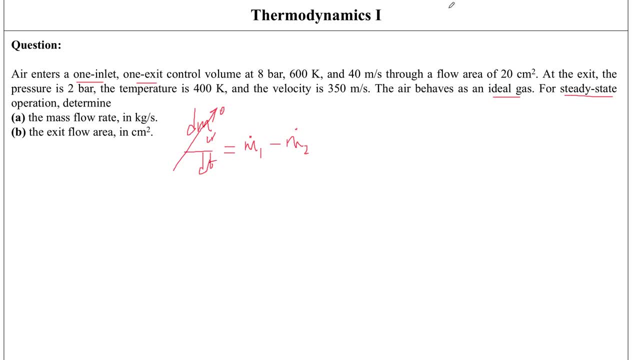 taking place according to time. Now again, try and construct a visualization of it. okay so, Okay. so now we're going to try and construct a visualization of it. okay, so you've got a control volume. you don't know what it looks like, so you can just. 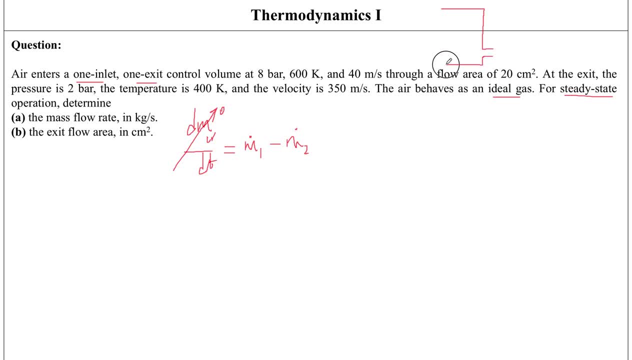 make it however you like, but you know that it's got one inlet and one exit, so that is what I'm gonna do here. okay, you've got one inlet and one exit. at the inlet, you've got conditions given to you eight bars, which is p1, and you got. 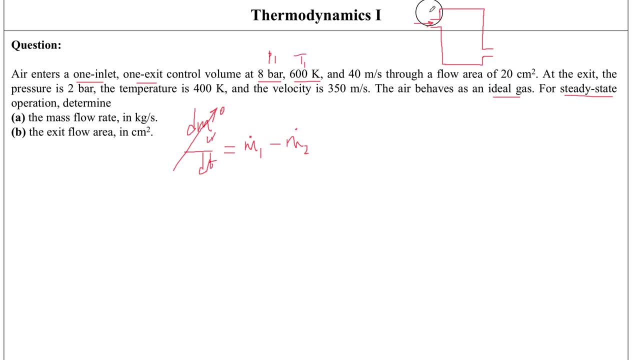 temperature given to you, which is t1. so this is your section one and this is your section two, which is the exit, and you've also got velocity given to you. okay, so you've got velocity given to you. I'm just gonna represent it by a different symbol, because we used symbol V for volume. so 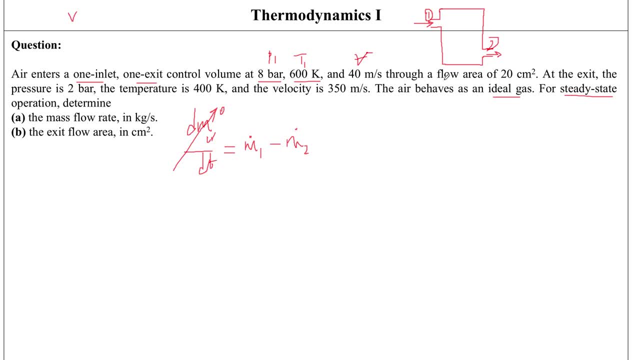 this is what I'm using. this is why I'm using a different symbol for it. you also got area given to you off this inlet and this is a area given to you off this inlet and this is a area given to you off this inlet and this is a. 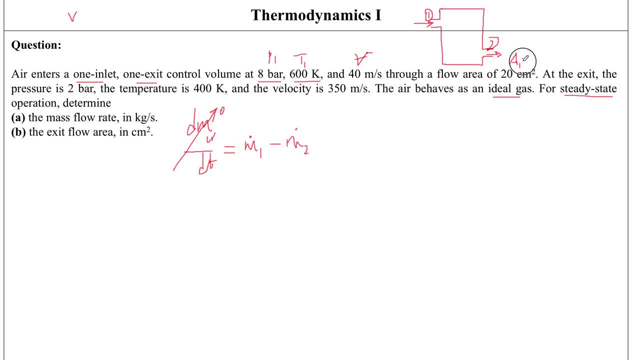 one. you can also write it in terms of meters square, so then it's gonna be zero point, zero, zero, two meter square. at the exit, you got pressure given to you, so this is P 2, and you've got a temperature given to you which is T 2 and the 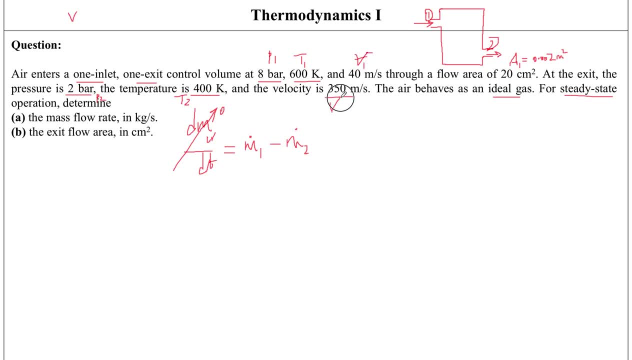 velocity given to you, this is V 1. and then this is going to velocity given to you, this is going to be V 2. okay, so you need to find out the be V 2. okay, so you need to find out the mass flow rate and you need to find out. 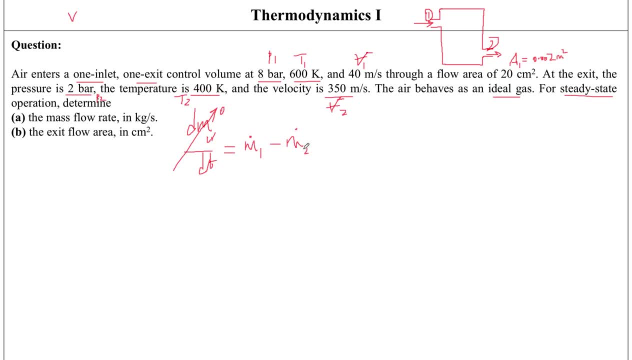 mass flow rate and you need to find out mass flow rate and you need to find out the exit flow area. so, because this goes, the exit flow area, so because this goes the exit flow area, so because this goes to zero, from here, M dot 1 is going to be. 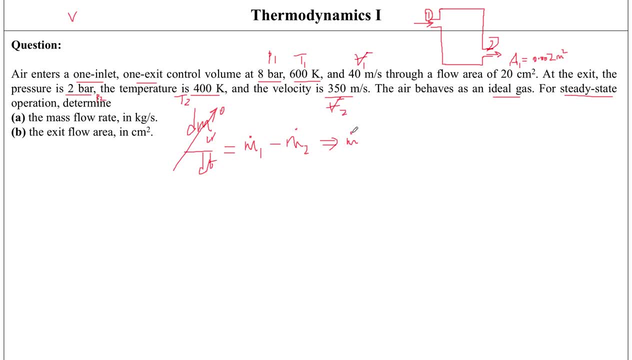 to zero. from here, M dot 1 is going to be to zero. from here, M dot 1 is going to be equal to M dot 2. or you can just write equal to M dot 2, or you can just write equal to M dot 2, or you can just write it as M dot, because M dot 1 is equal to. 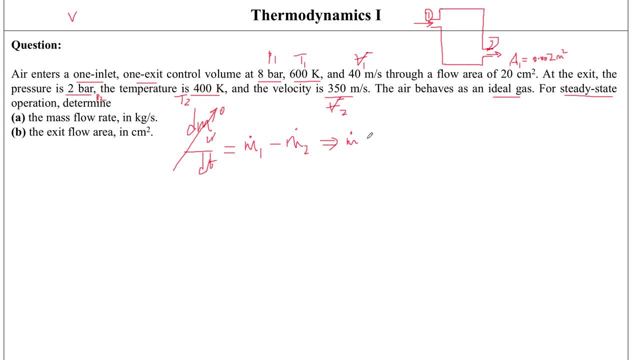 it as M dot because M dot 1 is equal to it as M dot, because M dot 1 is equal to M dot 2, which is equal to M dot. so how we're going to find this out? from the relationship rho a, b, because you already. 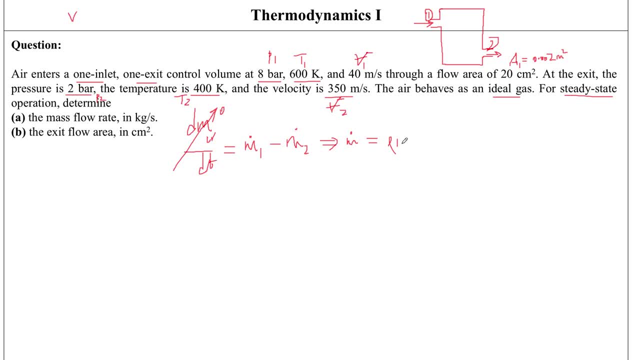 know that air is behaving as an ideal gas, so you can find out rho one. yeah, rho one area. you already have it as well, and the velocity at one. you got that too. so, and from the ideal gas law you can find out rho one, which is going to be. 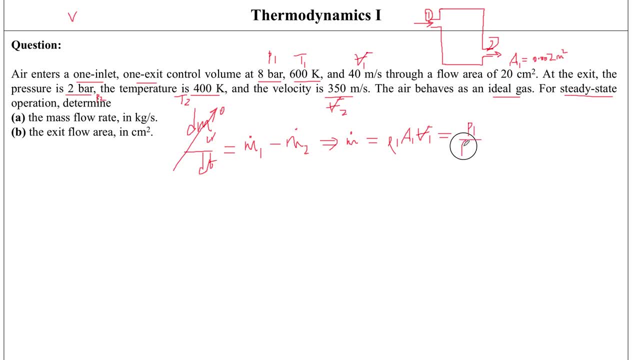 equal to p1 divided by rt1 and to area, which is given to you, at 1, and to velocity at 1. so obviously you're gonna have to convert pressure from bars into an appropriate unit. you're gonna have to find out this specific gas constant. so 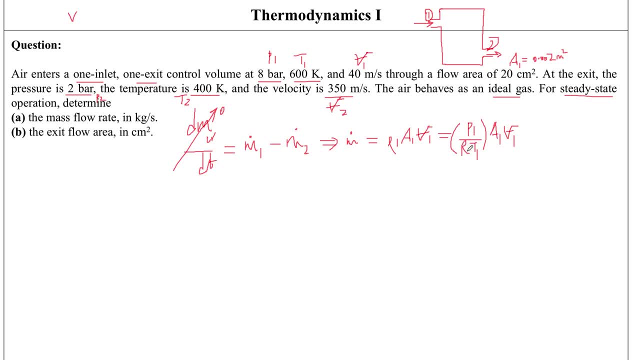 it's gonna be eight point three, one, four, divided by by 28.97- okay, which is for air- and just multiply it and you're going to be able to find out m dot from here. it's going to be around 0.36 kilogram per. 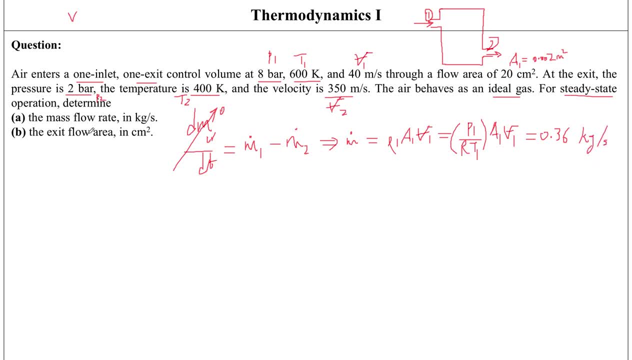 second. so now you've found out the mass flow rate. and now to find out the exo flow area, because you already know that m dot 1 is equal to m dot 2, so from here what that means is that row 1 a 1, V 1 is equal to row 2, a 2 and V 2 out of 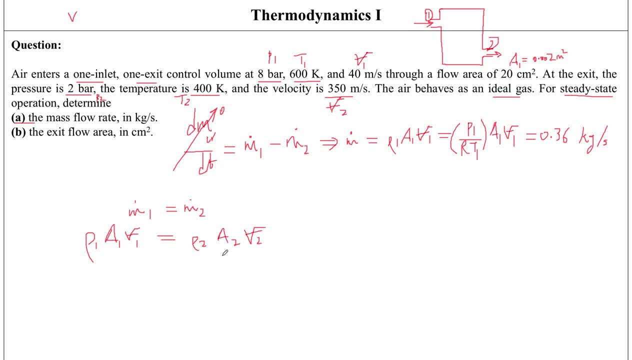 all of these, the only information that you don't know is a area 2, so you move all the other parameters onto the other side. it's going to be row 1 by row 2 into V 1, divided by V 2 into area 1 and now row 1. 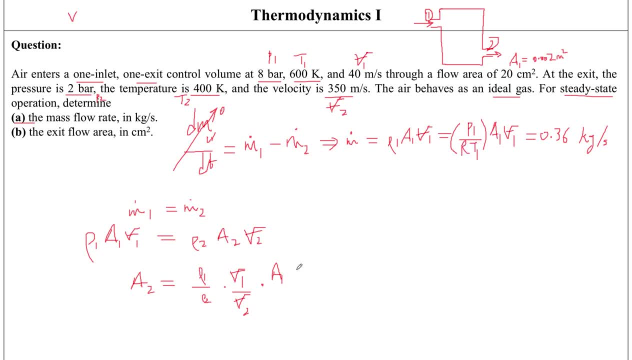 by row 2. everything is going to get cancelled out, except for pressures. okay, so it's going to be equal to 8 by 2: pressure at 1 by pressure at 2. 8 divided by 2 into: well, you also have, you're also going to have. 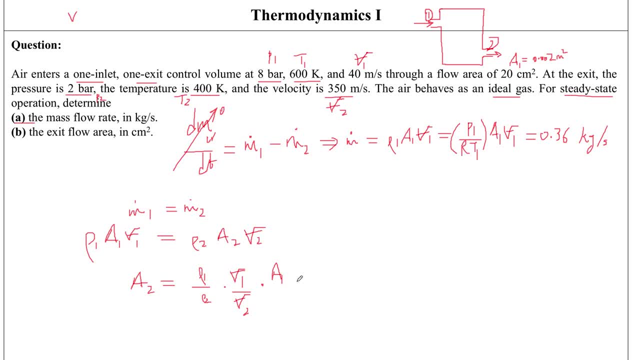 temperature as well. yeah, so let me just write this then, and it's going to be equal to P1 divided by P2, which are pressures, and then you're gonna have T2 divided by T1, and two velocities, V1 divided by V2, and two area at one. yeah, 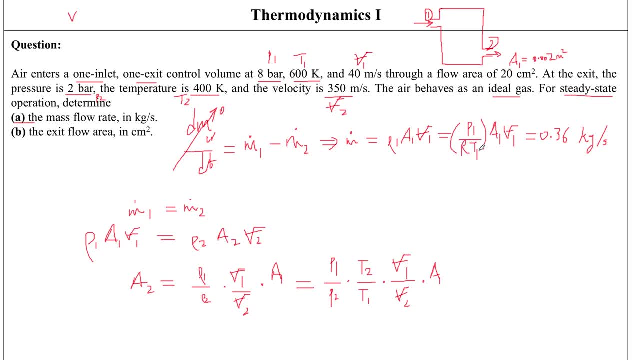 so R is gonna get cancelled out. obviously, you're gonna still have different temperatures that are given to your T1 and T2, so those are gonna stay in here and now this is gonna be equal to eight by two into four hundred by six, six hundred Kelvin's and Kelvin Kelvin's good- get cancelled out. and because these 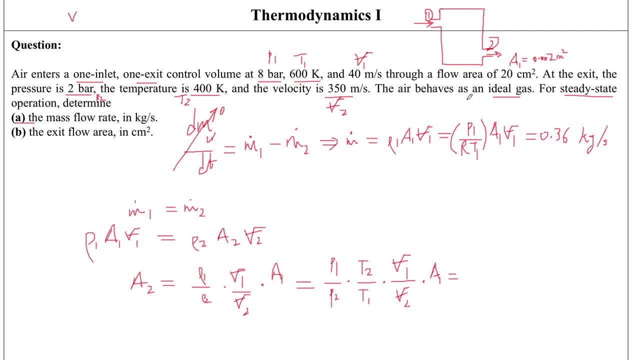 are ratios, and then you've got velocities: 40, 40 divided by 350, and then you've got area which is in centimeter square. just leave it in centimeter square. so you're gonna find out area two in centimeter squares as well, and that's gonna be equal to around. 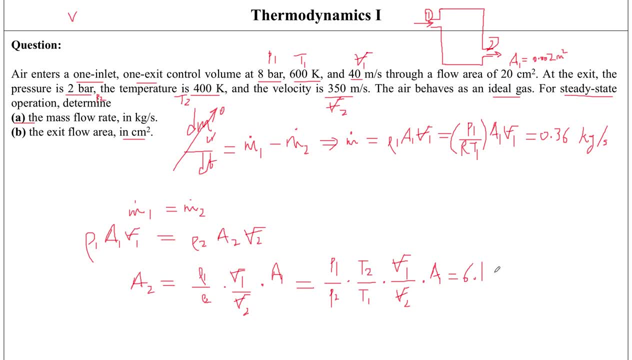 six point one centimeter square. so this is how you've been able to apply the conservation of mass principle for a control volume, and now we're gonna move on to looking at a couple of examples where we not only apply the conservation of mass principle, but also apply the conservation of energy principle as well. 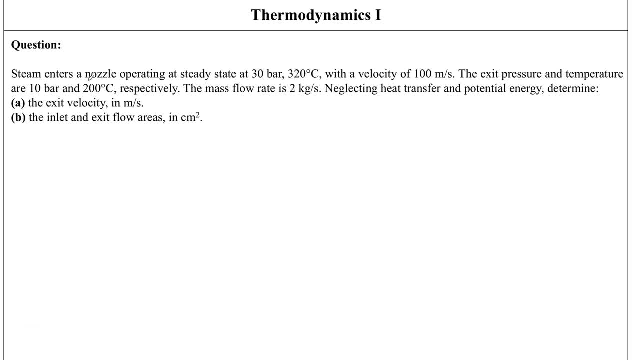 so this is a question: where you've got steam that is entering into a nozzle, you already been told that it's operating in steady states of. so the time terms, the change according to time terms, are going to disappear in both the mass balance and, if you were to apply a cause of concentrationwolf, the change according to time terms. 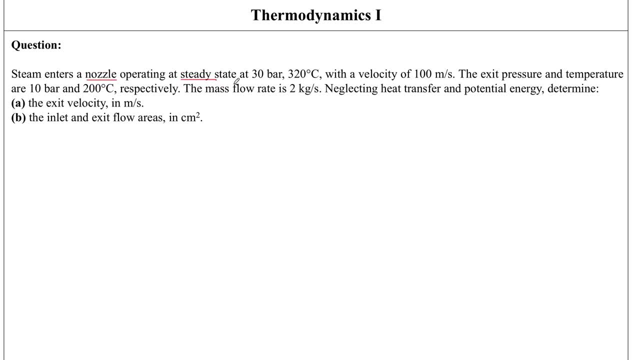 are going to disappear and both the mass balance and, if you were to apply a nieahr of high weather circle, intr烯 and high grader大家好- the conservation of energy as well. you've got information given to you at the inlet. you've got the exit information given to you: mass flow rate. 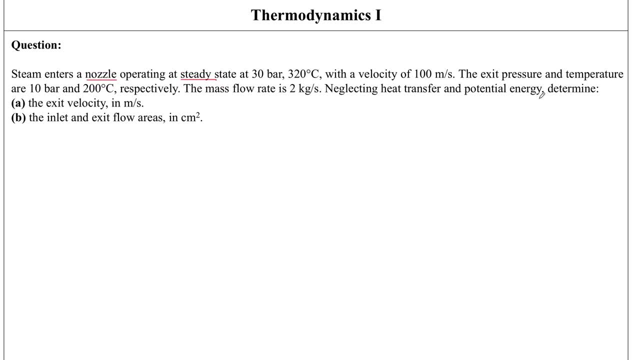 that is given to you, you're neglecting heat transfer and potential energy changes, and you have to find out the exit velocity and the inlet and exit flow area. so, again, because you're talking about a nozzle, you don't know what kind of nozzle it is, so I'm just gonna make a nozzle, which is: this is a. 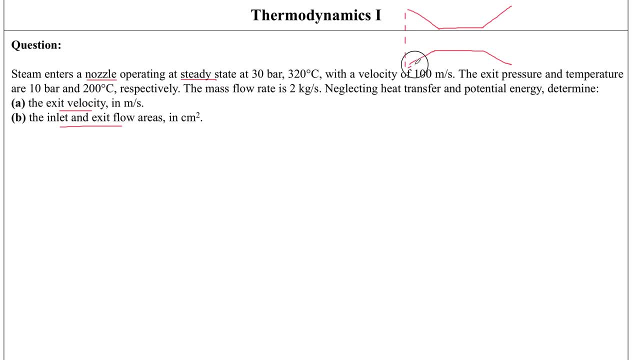 CD nozzle, and obviously we don't know what kind of nozzle we're using. it could be a converging nozzle as well, but so you've got your nozzle and now you're making the boundary of the system. okay so- because this is something that we've discussed as well- that you can have imaginary boundaries of the system as. 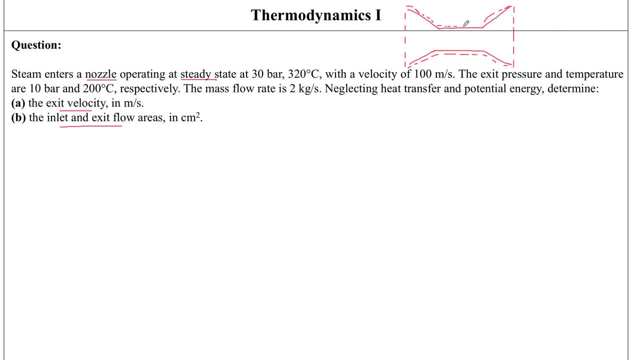 well, where you don't really see any inlets or outlets. so over here, got imaginary boundaries and, Machdin, you've got this as your inlet, you got this as your outlet and this is your, basically, section 1 off the flow and this is your section two of the flow. 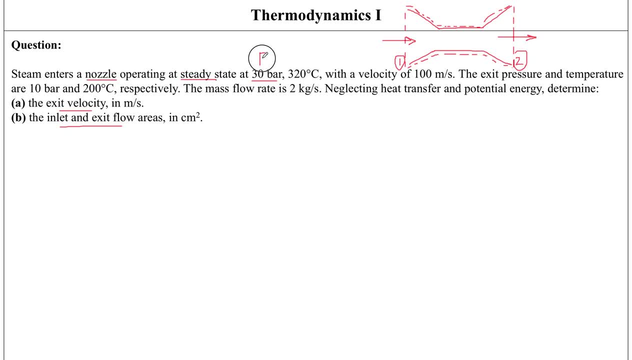 and one. you've got 30 bars of p1, you've got the temperature, which is T1, and you got the velocity, which is gonna be V1, and at the exit, you've got pressure given to you, which is p2, temperature given to you, which is T2, okay, And you've got mass flow rate that is given to you. so this is. 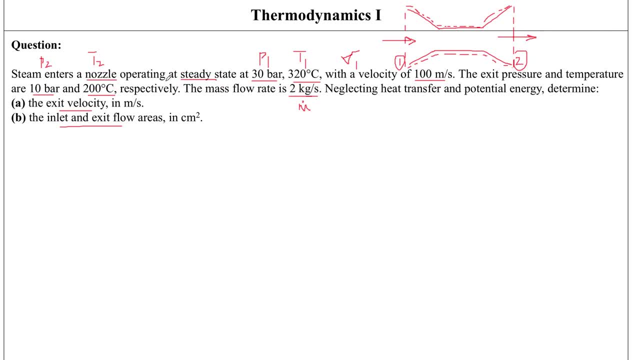 going to be m dot. So because we're talking about steady state, that means when we're looking at the mass conservation equation, obviously that term is going to go out dm over dt. that's going to disappear and m1 is going to be equal to m2, and then that is equal to m dot. okay, So that's. 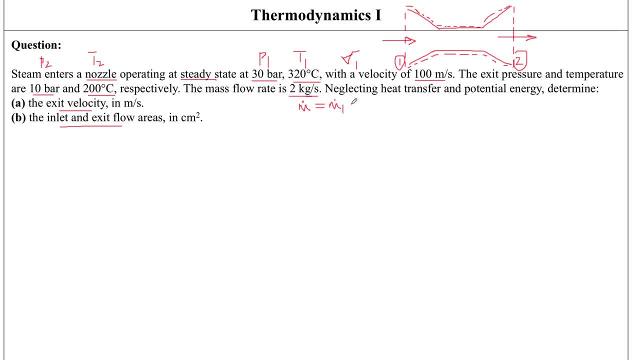 how we've got a constant mass flow rate, because m dot 1 is equal to m dot 2, which is equal to m dot, just like in the previous question. And now we can go ahead and apply the conservation of energy principle onto it, the energy balance, and I'm just going to write the full equation: 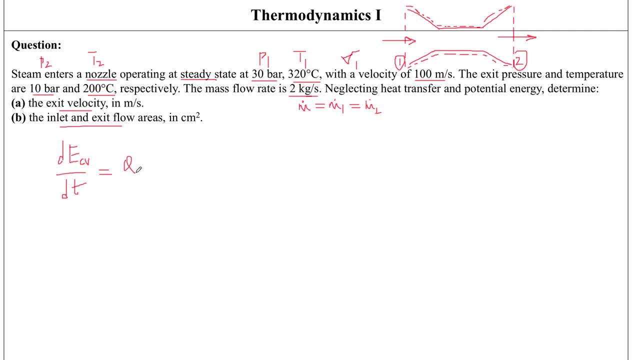 and then we're going to go step by step and eliminate the energy balance. Well, we can, based on the information that is given to us. okay, So you've got work done across the control volume, and then because your mass flow rate is constant. so that's why m dot is. 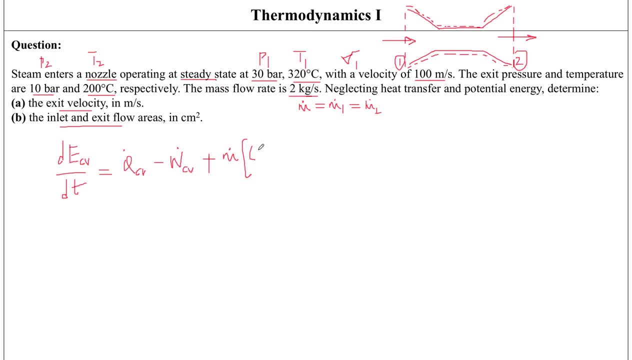 going to be applied on the change in, let's say, enthalpy, or the change that you see for energy conservation, Kinetic energy. so that's going to be v1 squared divided by 2, or you can just do the whole thing. 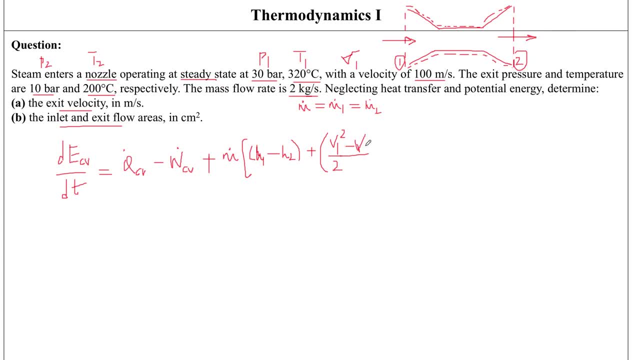 instead of just writing it like that. So v1 squared minus v2 squared divided by 2, plus you've got the potential energy changes, which are going to be gravitational force or like actually gravitational oscillation acceleration, sorry, into Z1 minus Z2.. 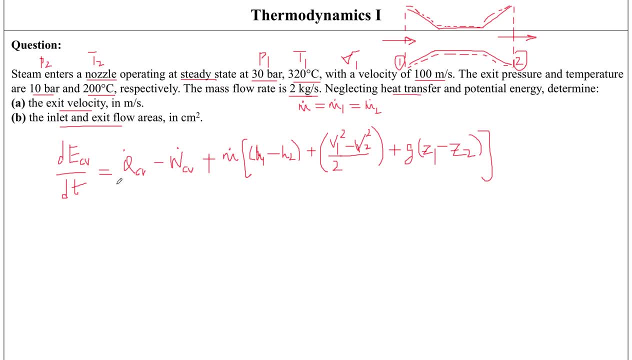 So, from here, you're neglecting heat transfer. That's why this is going to go out. But, most importantly, this is going to go out because this entire process is taking place at a steady state, And a steady state, this is what we mean. This goes out. 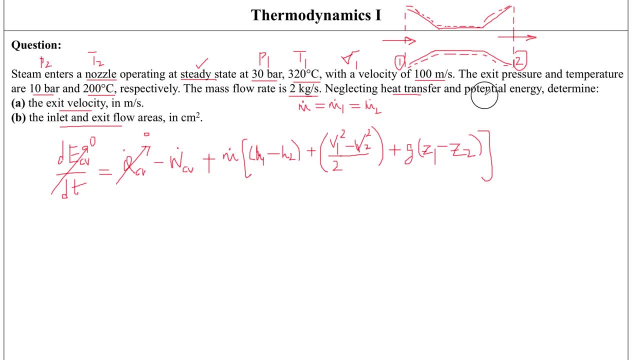 Heat transfer goes out. You've got no potential energy changes, so you're neglecting that too. So this is going to go out. And then this is also going to go out because for a nozzle like we've seen in one of my previous videos, and I'm going to leave the link for it over here- 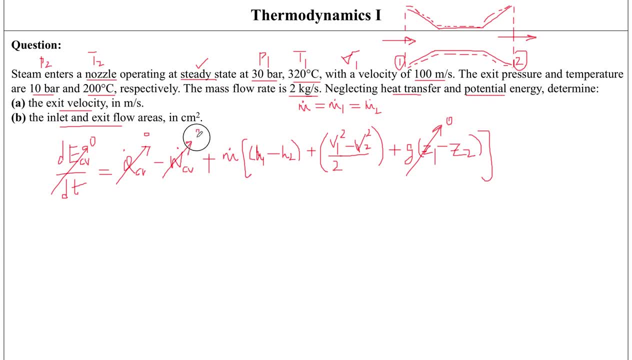 that for a nozzle, there is no work across the control volume, Okay. so that is something that we need to be mindful of as well, And now that we've got all of this left, we can basically see the knowns and unknowns here. So you've got m-dot, which you already know. 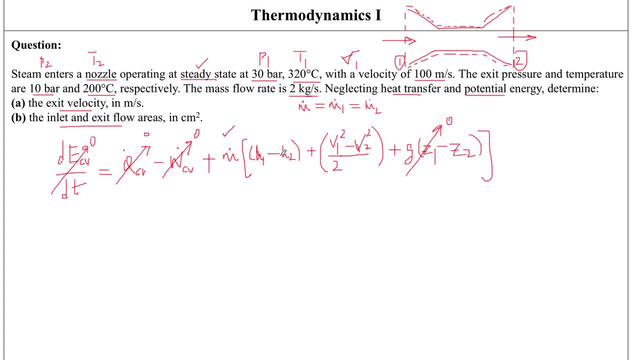 Enthalpy information H1 and H2, how are you going to find that out? You're going to go to the tables. You already have the pressure temperature information at both the points, at both the sections. So that's why you can find out H1 and H2 from the tables. You've got velocity given to you. 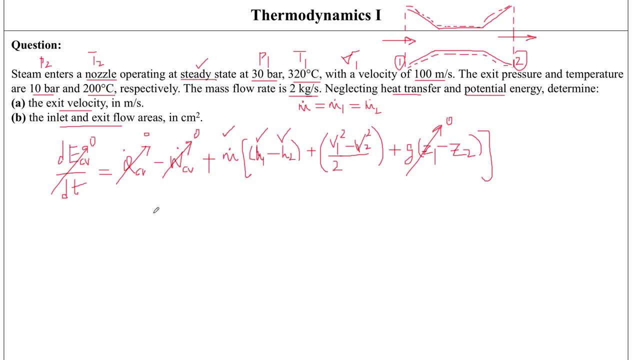 at the inlet. So from here you can find out the exit velocity. Okay, so V2, if you simplify this, it's going to be equal to 2 into H1 minus H2 plus V1 square, and this entire thing is going to be. 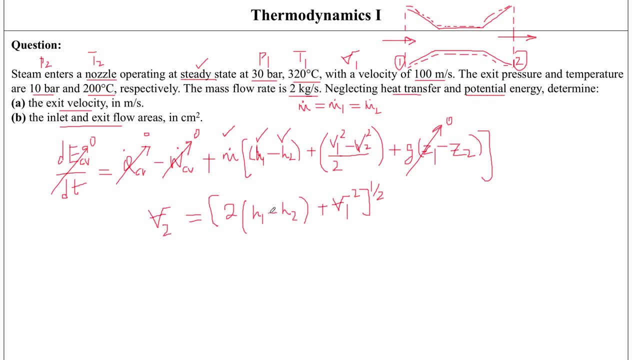 under root. So we've got V2 that you can work out from here. Just to give you more hint about how to find out H1 and H2, you can go to table A4 because you're dealing with steam, so water. 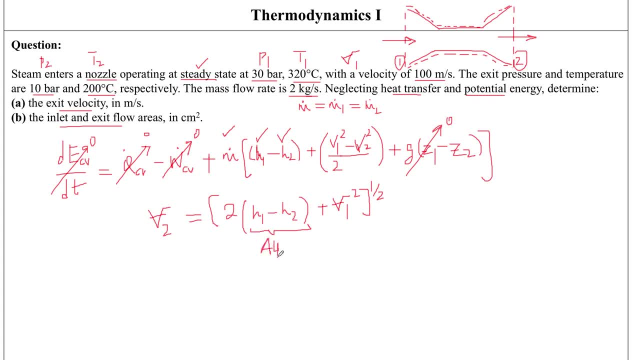 So you go to table A4 and from there you start finding out H1 and H2.. Once you know those two, you can go ahead and plug them in here. You already know V1, so you're going to be able to find V2.. I'm just going to give you an approximate answer so you can check your answer against it. 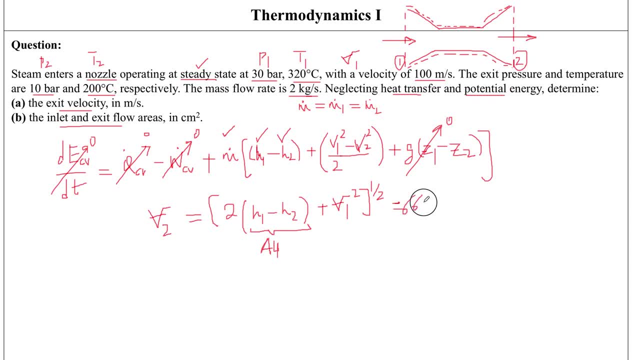 It's going to be around V1.. So you're going to be able to find V2.. I'm just going to give you an approximate answer so you can check your answer against it. It's going to be around 660 meters per second. 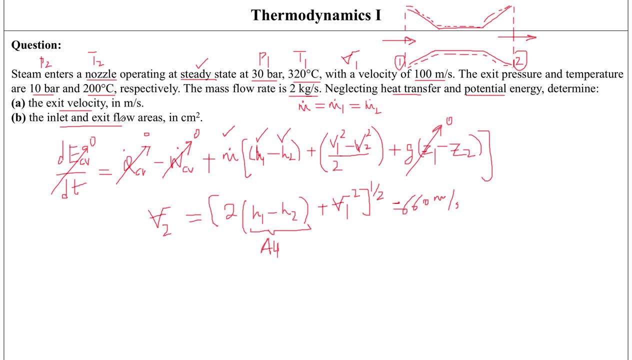 Okay, now you got this, You can. you can go ahead and find out the inlet and exit flow areas. Now, you're going to do that because m dot is equal to area into velocity divided by specific volume. So from here, you can go ahead and use this exact same relationship for m dot. 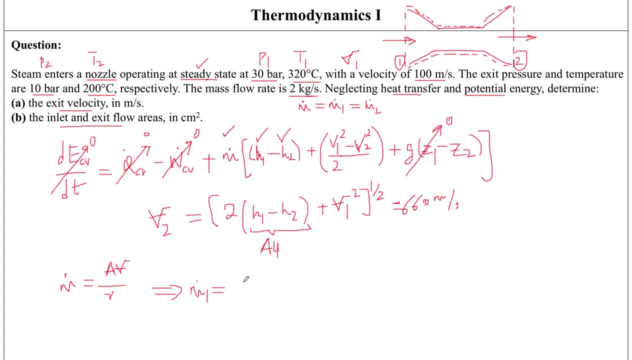 So you've got one. Okay, we're just going to give you area at 1 and 2.. Velocity at 1 divided by specific volume at 1. And from here you can find out the area at the inlet. Okay, and you can just plug these in again. You've got to find out the specific volume from the tables. 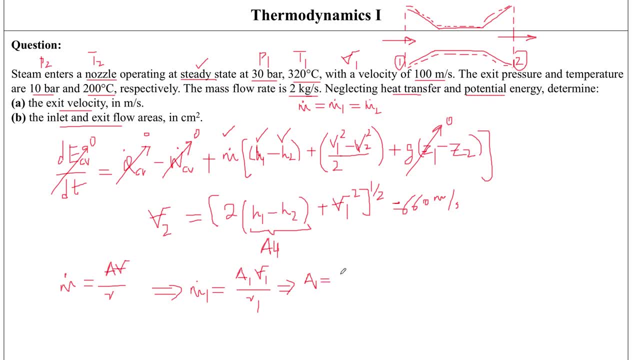 and you can go ahead and do that yourself. this is going to be around 16.6 centimeter square, okay, area at one, and just like this you're going to use hold on, I'm going to use the relationship or M dot 2, and from here you're going to find out area at 2, and that's going to be around 6. 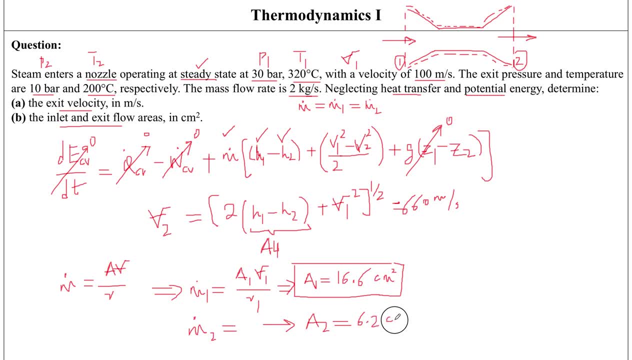 point 2 centimeter square, so you can go ahead and check these out yourself. and now we're going to move on to another problem. it's going to be a bit more complicated. so we're going up in the difficulty level from problem 1 to 2 to 3, and now we're on the other side. we're going to unlikely. 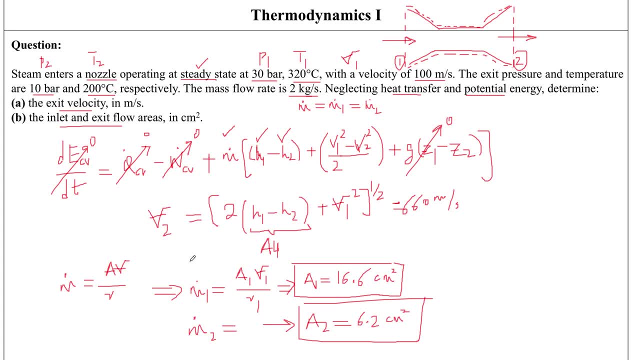 anything for x plus 2. so we'll be the same for long term, so that فث and y niew park these a little for, and that's going to be about applying both the conservation of mass and conservation of energy principle as well for a controlled volume. 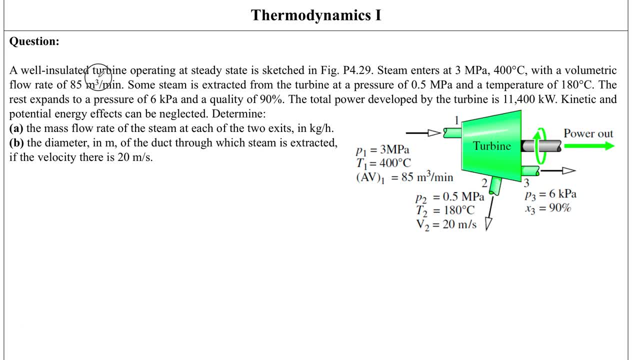 Okay, so you've got a turbine. Again, start off with what you know. You've got a turbine that's operating at a steady state- This is the figure for it. You've got conditions given to you at the inlet and you've got steam that is being extracted from the turbine and the rest is being. 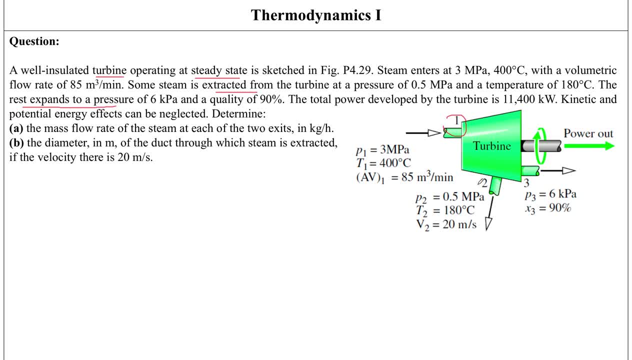 allowed to expand separately. Okay, so you've got one inlet, you've got two outlets, then you also got total power that is being developed by the turbine. Okay, so that's over here, power out. and that is your work, done by the control volume. 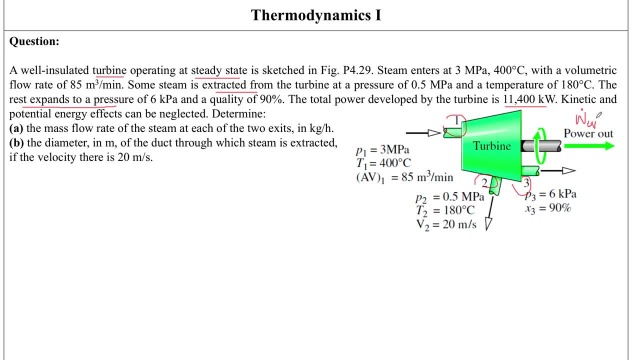 Okay, so this is being developed by the turbine. You're neglecting the kinetic and potential energy effects. You have to find out the mass flow rate of the steam at both the exits. You've got to find out the diameter as well. So you need to first of all see what you need to find out. 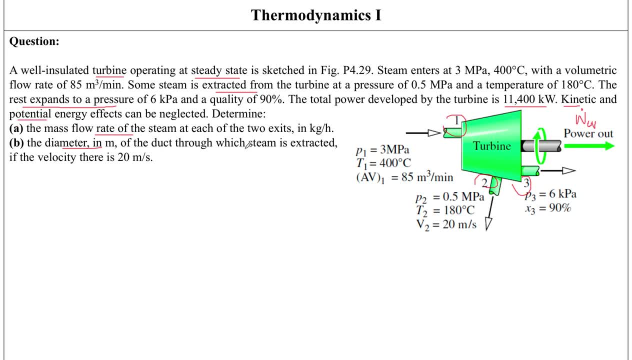 and then go ahead and apply the conservation of mass or conservation of energy principle on it or both. You shouldn't just start applying the conservation of mass principle onto any control volume, because you need to see first of all what is being happening underneath the turbine. 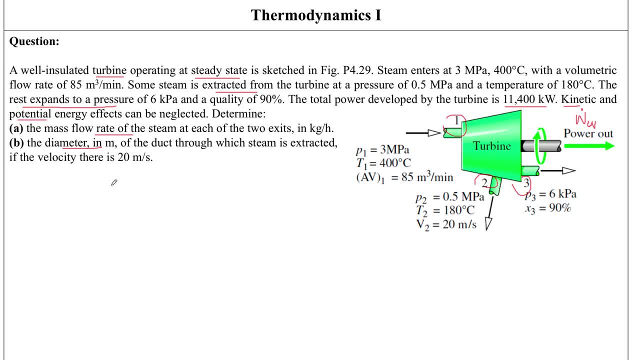 but then also before, appears as something sudden that lines are closing into a contro groom. what's the information that you're being told to find out? So, if you apply the mass rate balance on it, because it's operating in steady state, so the left-hand side is going to be 0, and the 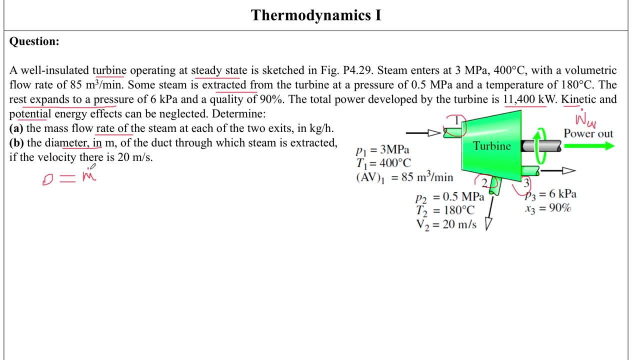 right-hand side is going to be, because you only got one inlet, so m.1,. you got two outlets, so minus all outlets, mass flow rate at all outlets. so it's going to be m.2 minus m.3, okay. 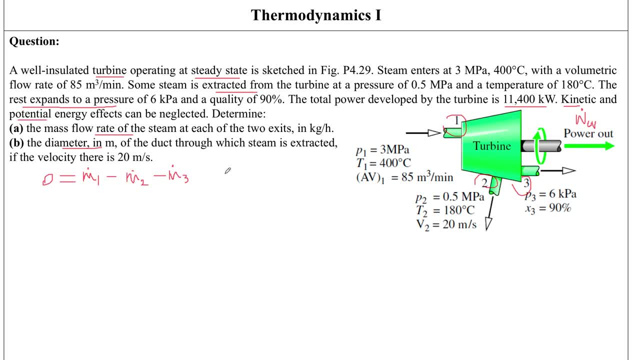 And I'll just leave it at that for now, and let's call this 1, equation 1.. Actually, you can also find out m.1 here, and the way to do that is because you need to see the information that is. 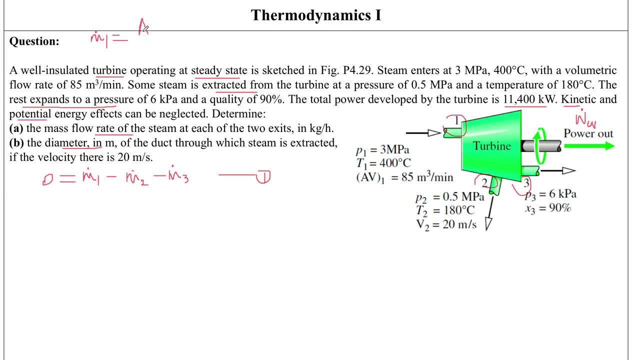 given to you. so m.1 is equal to av1, okay, av at 1, and this is called what It is called, the volumetric flow rate. Okay, so volumetric flow rate divided by specific volume at 1 is going to be equal to. you've got. 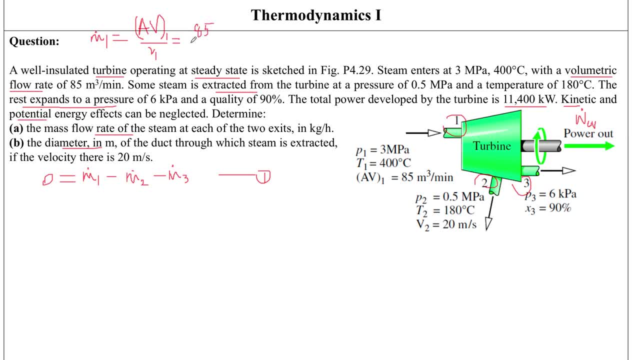 85 m3 per minute divided by that specific volume here that you need to find out, and you can find it out. and how do you know that? You've got temperature and pressure information given to you. so you can go ahead into the tables and I'll give you a hint. go to table A4,. 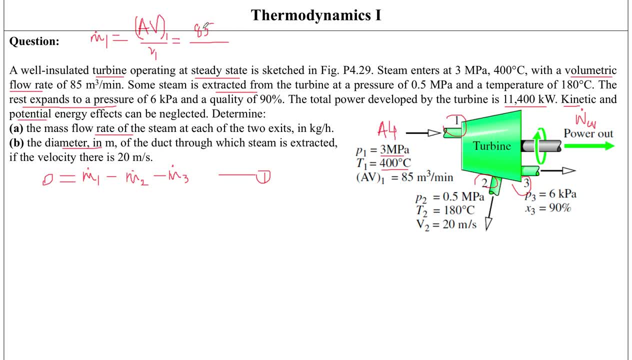 and find out the specific volume at 1.. So you're going to have to work with the units here as well, because this is in meter cubed per minute, and then the specific volume that you're going to find out is going to be equal to some value in meter cubed per kilogram. so once you find that, 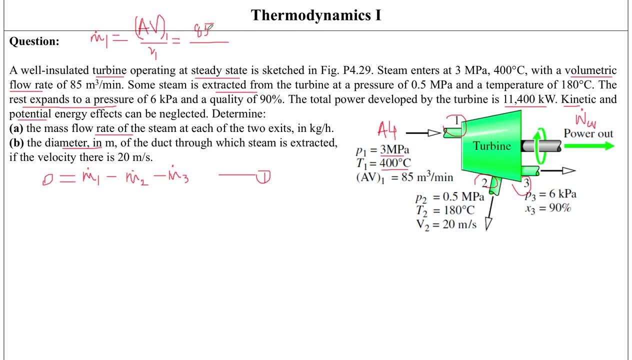 out, plug it in, change the units for it and I'll just tell you what v1 is so you can compare it. 6.0, 9.94 is going to be equal to 14.2 kilograms per second. so you've got m1 that you found out, m.2. 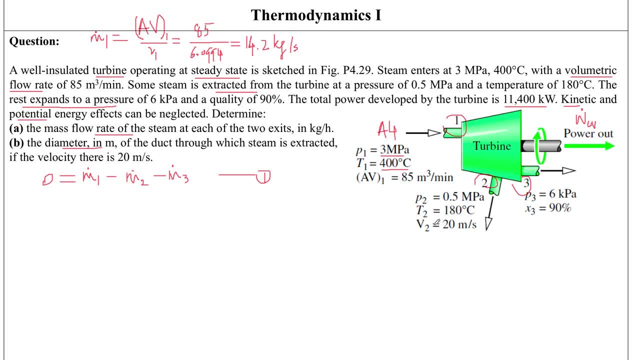 you can't find out because you've only got velocity information m.3 you can't find out as well. so because we can't find it out, we're going to have to go to the energy rate balance and again the left-hand side is going. 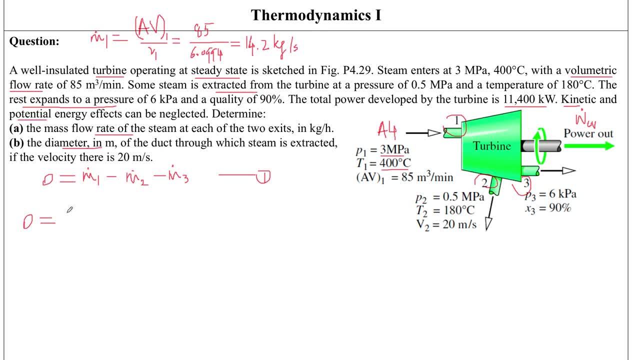 to be equal to 0 dE by dt and it's going to be equal to q dot: heat transfer across the control volume minus work done across the control volume plus m dot. and now, because m.1 is not equal to m.2,, 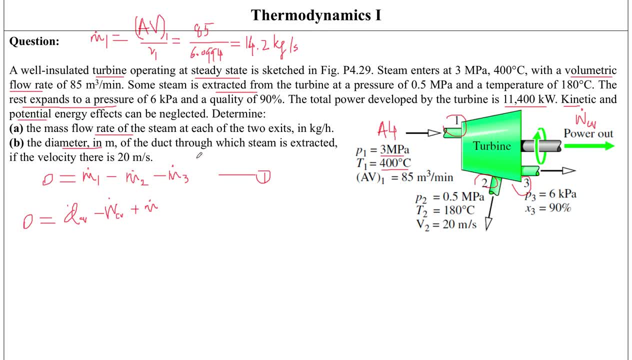 so we're going to have to go to the energy rate balance and again, the left-hand side is going to be equal to m.2, because if you were to write this, let's say, you could write it in terms of m.3,, one of the outlets. 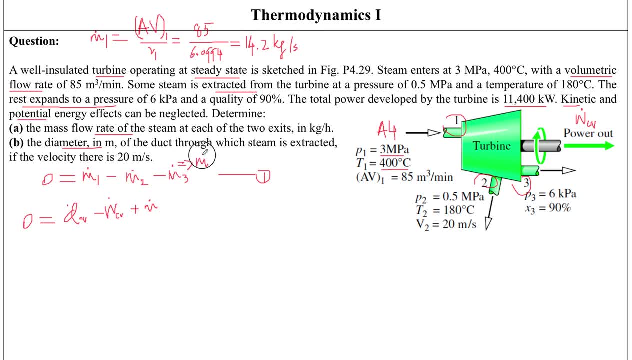 and that's going to be m.1 minus m.2, so because you can't combine all of them and write it as m.1 into you, can't write it as m.2 into m.2, so you're going to have to go to the energy rate balance and again the left-hand side is going to be equal to m.2,. 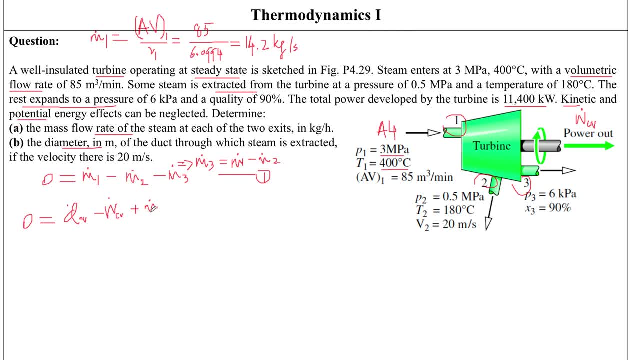 the entire thing, like we did in the previous question. so m.1 is going to have its own separate set, which is going to be h1 plus v1, squared divided by 2, plus gz1,. okay, and just like that. this is for m.1, just like that. actually, it's going to be a minus here. 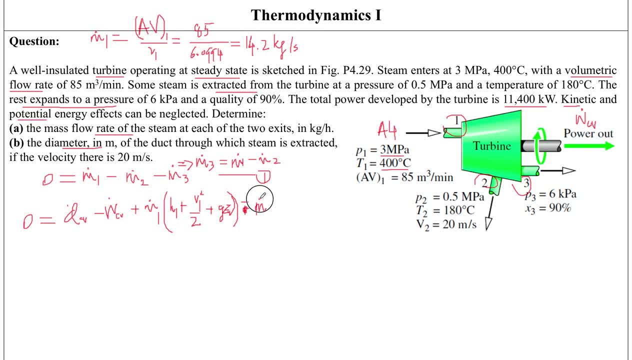 now because you're talking about the outlets. so m.2 into the entire thing. but I don't need to write the entire thing because I already know that the kinetic energy effects are being neglected, the potential energy effects are being neglected, and I can go ahead and just write minus m.2 into. 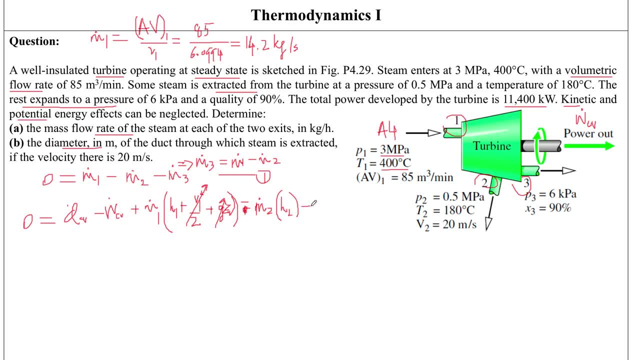 h2 minus m.3 into h3, okay, what else? because I've got no information given to me by which I can determine heat transfer rate, or it's not specified simply in some way that like how the work done is being specified. 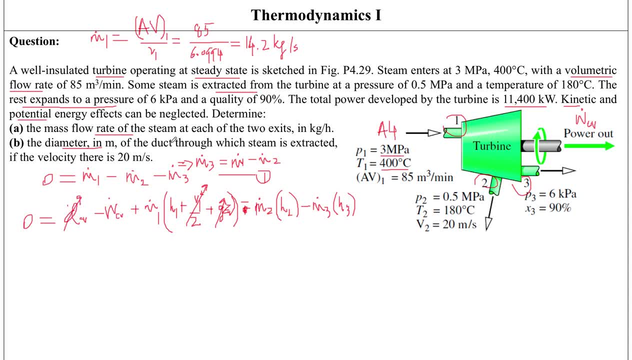 that's why I can just neglect that as well. unless there was- let's say there were- some values given here through which I could have found this out, then it wouldn't be zero. okay, this goes to zero. and now you've got. zero is equal to minus work done across the 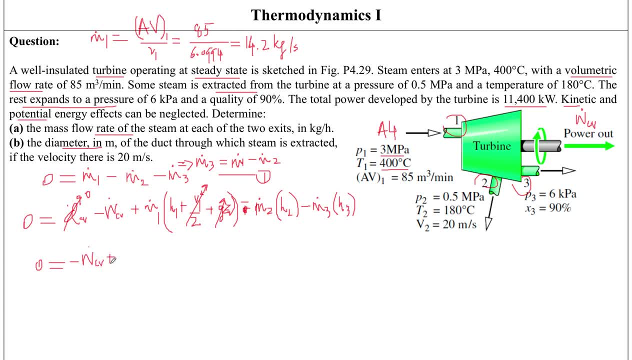 control volume: plus m.1 into h1, minus m.2 into h2, minus m.3 into h3, over here you already know what m.1 is. so you've got two unknowns here and when you've got two unknowns. that is why you needed another equation for two unknowns. 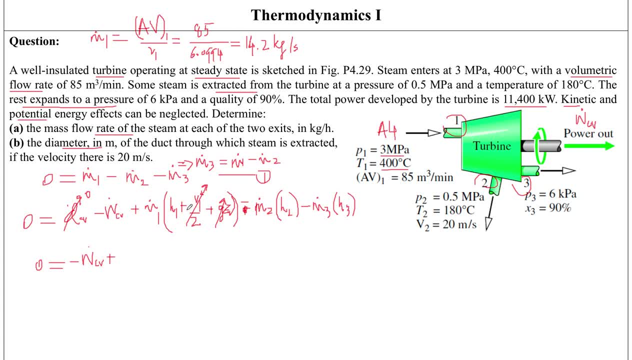 you need two equations. you've got one equation, which is this, and from here you can have the second equation, because you already know what m.1 is into h1 minus m.2 into h2, and then, instead of writing m.3,, you can write it in terms of m.1 minus m.2, so just plug that in here. 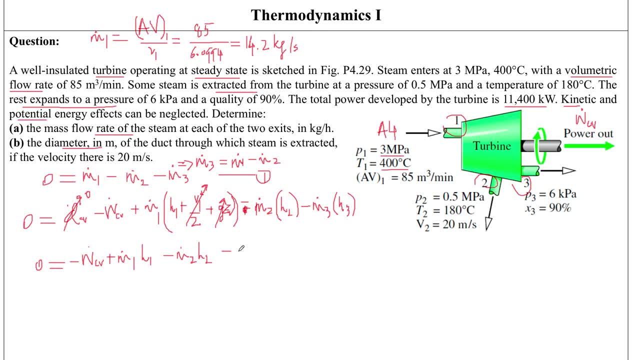 it's going to be minus m.1 into h3, plus m.2 into h3, right, so you just plugged in the value of m.3 here from this equation. okay, once you've done that, you can simplify it now, because 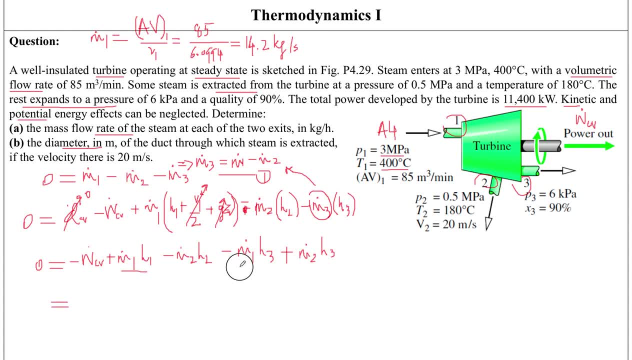 on this side. you've got m.1 h1, you can take this out, and you've got m.2 h2, m.2 h3, so from here you can simplify it even further by writing it as m.1 into. you can take it out as a factor. 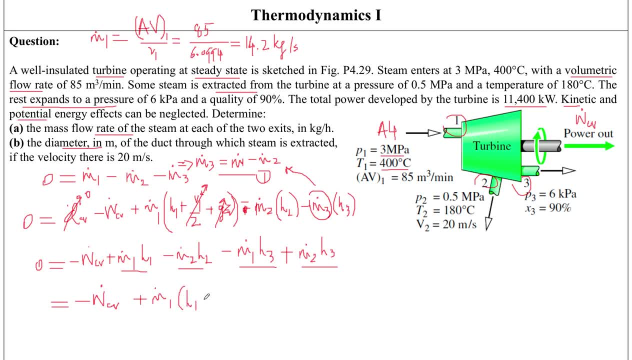 and then m.1 into h1 minus h 3, this is 3, minus m.2 into h2 minus h3, okay, this is equal to 0, so the information here for h1 and h2, you can find them out from the tables directly. okay, just go to table. 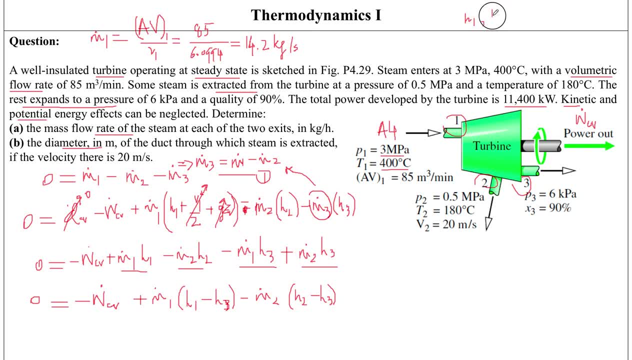 A3, and you can find out h1 and h2 from table A3, but for h3, you need to be careful about it because you've got quality already given to you and that means that it is a mixture. so for when it comes to mixtures, then you have to apply the equation h3 is equal to hf. 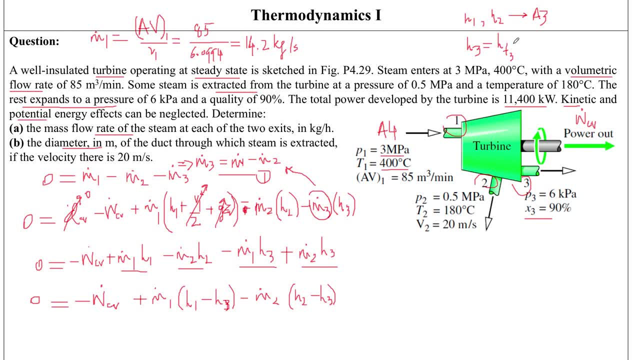 at 3,. so you find this out from the table, plus x3,, which is quality 90%, 0.90, into hfg at 3,, and this is something you find from the table as well. so you find out the values for h1,, h2, and h3 from the tables you already 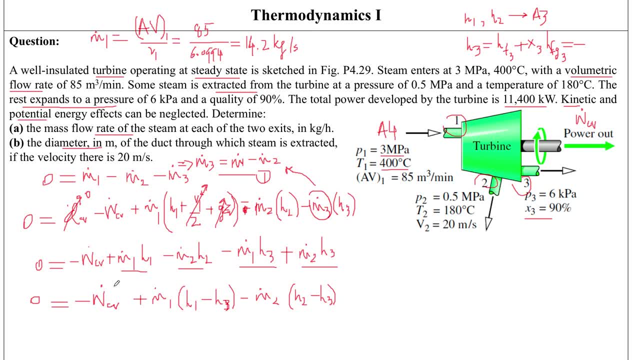 know what m.1 is, you know what working across the control volume is, so you can find out m.2 from here. right, so you can find out m.2 in terms of working across the control volume: mass flow rate at 1 into h1 minus h3, divided by h2 minus h3, which will be multiplied by m.2,. 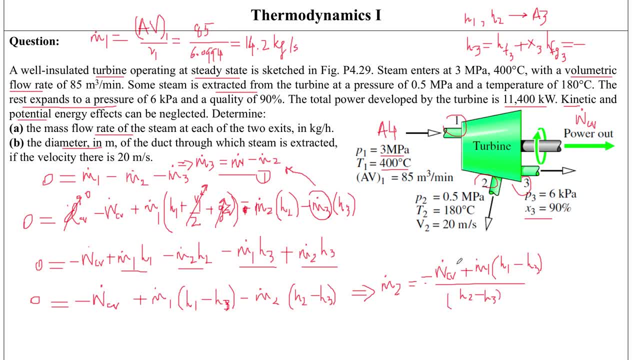 okay, so you've got m.2 that you found out from here and I'm just going to write down what the value is going to be so you can compare- and it's going to be around 3 kilograms per second and you've got. 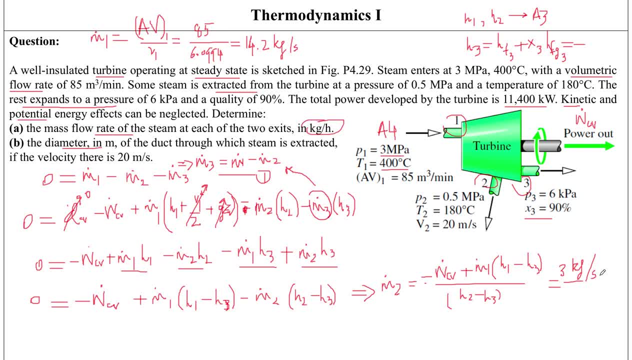 to convert it into kilogram per hour, because that is what's being asked. so you can do that yourself, and from here you can find out the value for m.3 as well, because now you know m.1, and m.2, and m.3 is going to be equal to. 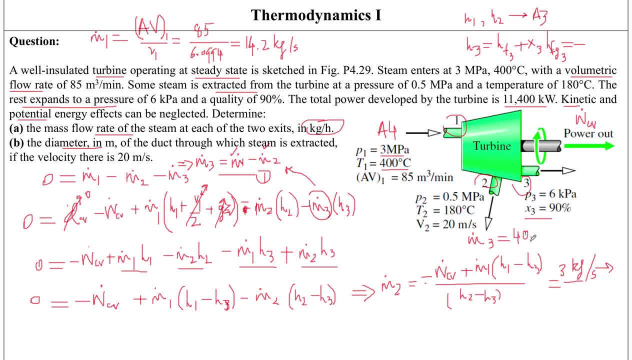 I'm going to write this and you can check it out for yourself. kilogram per hour, okay, so you're going to have to check these out yourself, and we also need to find out the diameter now, so to which the stream. 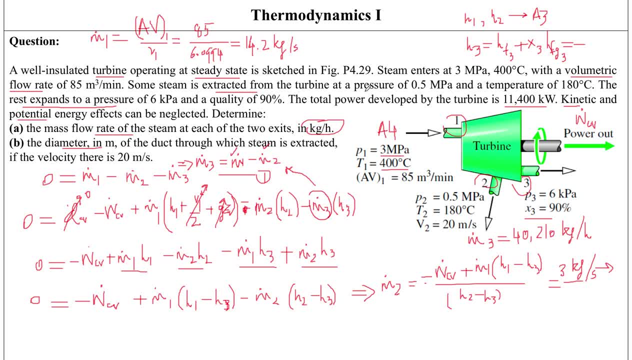 being extracted and we're extracting the steam at state 2. so we need to find out the diameter here and to do that, I'm gonna do it like we saw in the previous question: find out the area at 2, because the mass flow rate information at 2 is. 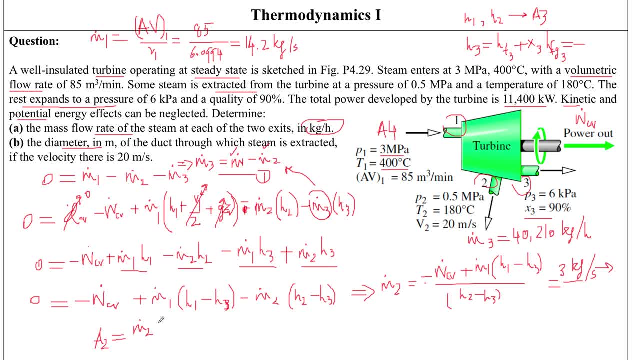 given to us. specific volume is something that we can find out as well. so that is going to be V 2 divided by velocity at 2. okay, from here you can find out the area. at 2, it's going to be around 0.06, 1 meter square, and now that you have the 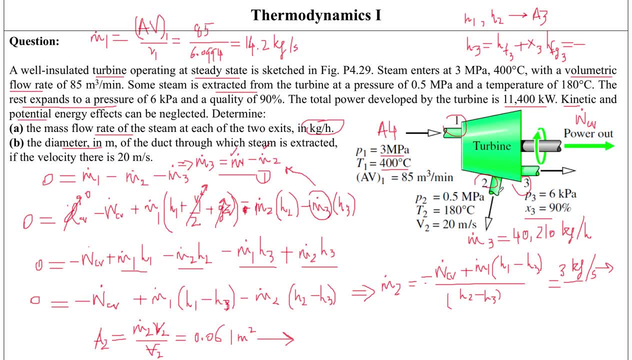 area. you can go ahead and find out the diameter as well, because it's a circular cross-section, so that's going to be square by 4 and then diameter is going to be equal to 4 into a 2 divided by pi under the root. okay, that's going to be equal. to find it out yourself and check. 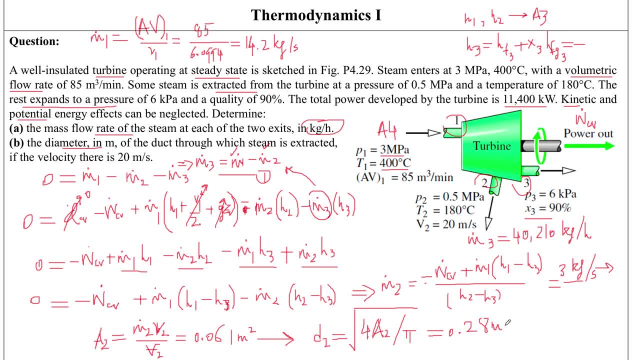 it from here, it's going to be equal to 0.28 meters. so that is how you solve a 경제에 대한 변화가 있습니다 and you can do. you can get a lot of different questions related to control volume analysis. control volumes, mass can. 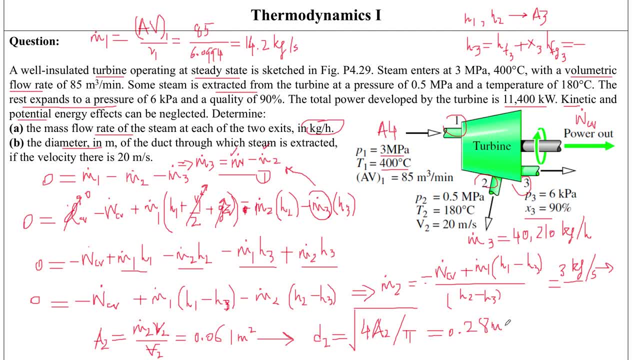 flow into and out of system. energy changes can take place for the system and you need to start from the very basics. you need to see, depending on what kind of question you're solving, depending on how many inlets and outlets you've got that- how you can solve that kind of question. okay, so this is just to.